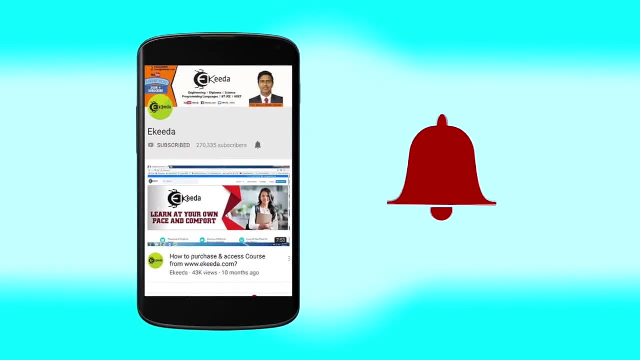 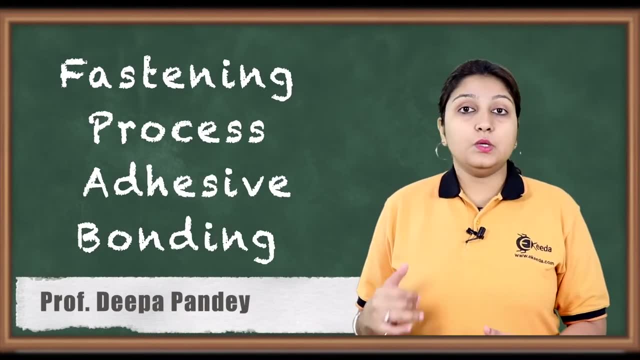 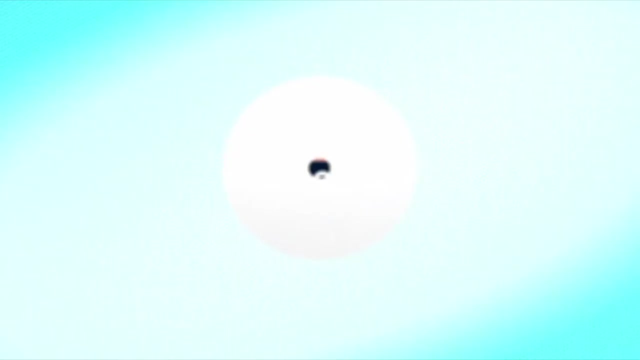 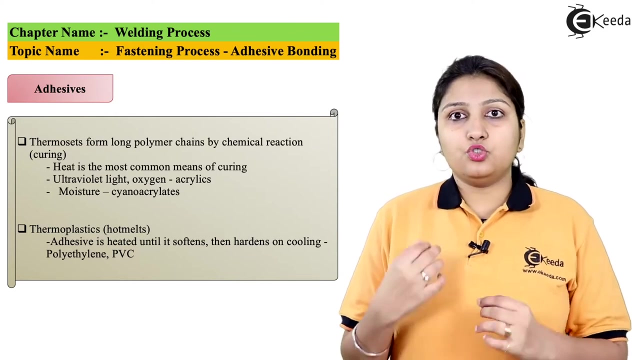 Click the bell icon to get latest videos from eKIDA. So, as I've told you what are adhesives, If you are seeing a glue, it is an adhesive. It is used to join the paper or any other object, like your cardboard or any other thing. It is a kind of 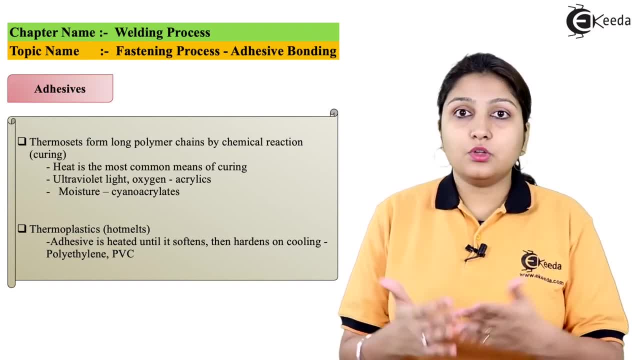 adhesive. So it is a kind of joining process. You're joining to papers or you're joining to cardboard. Same way, any other chemically active adhesive can be used, like epoxy or resin or any other thing can be used again and again for your joining purpose. So adhesive can be thermosets. 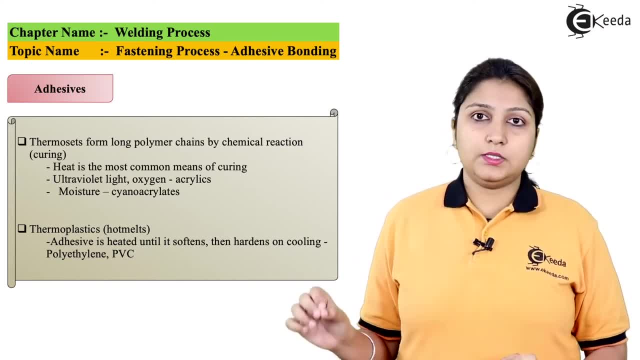 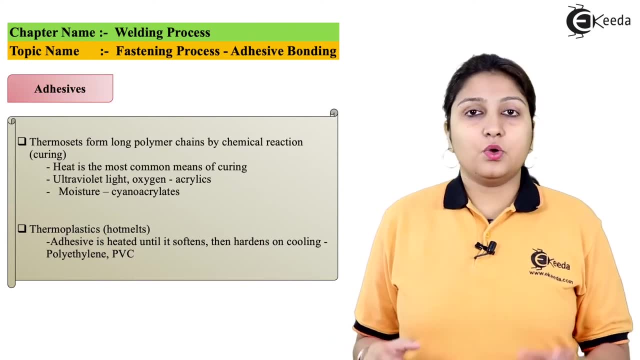 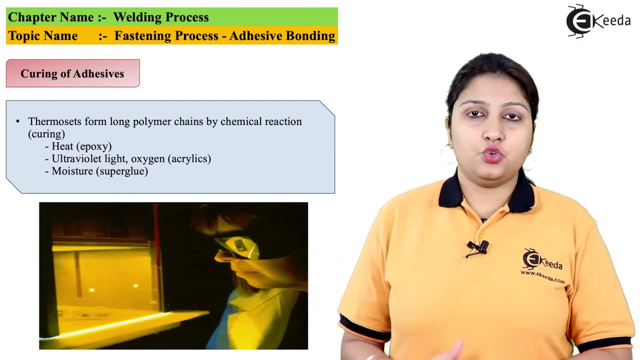 or it can be thermoplastics. In thermosets the exact heating can be done through curing and in thermoplastic heating can be done by just melting it. So how it is done we'll be seeing in our next slide. So in this diagram you can see a curing part is being shown, The worker which 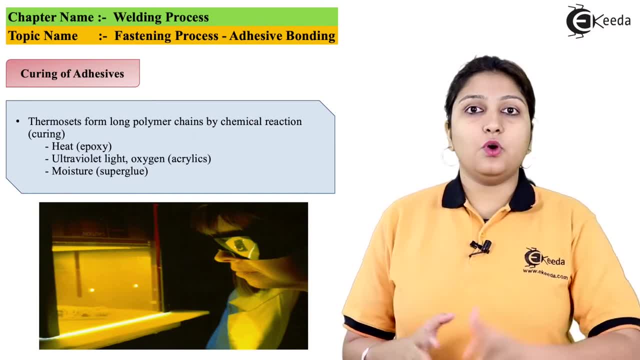 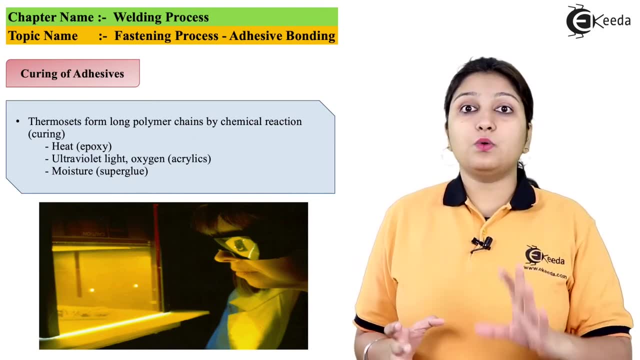 is there. what you have to do is you just have to keep your adhesive part, like your metal, which is adhesed already. You have to keep it inside and what you have to do? you just have to see how it is curing. So what you have to do is you just have to keep your adhesive part, like your. 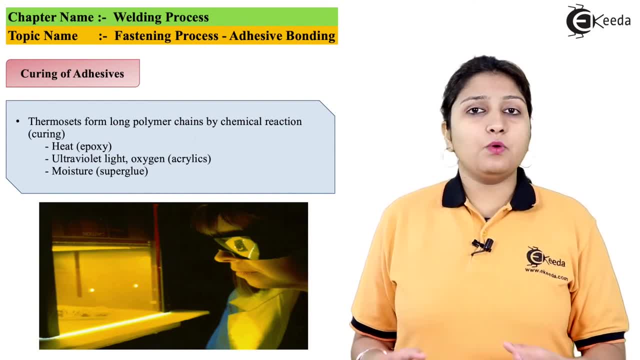 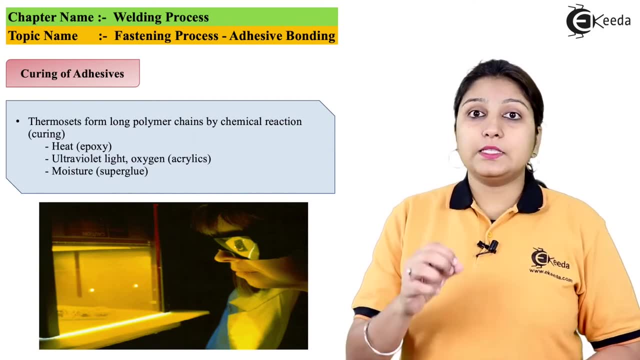 metal which is adhesed already, You have to keep your adhesive part. like your metal which is done, Heat is applied, additional some amount of moisture is given and curing is done. So after applying your adhesive on the object, exact curing is done just to set your adhesed part. So if a 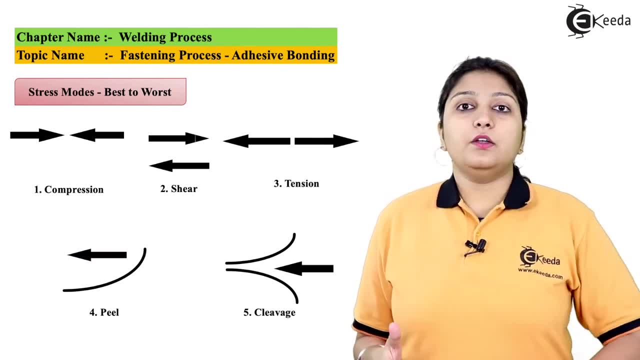 part which is joined by adhesive bonding, such kind of stresses occur. I have just named some 5 types of stresses. One is compression: It can be compressed, Sheer. shear means part to part reaction, like it can be sheared, like this. third one is tension: it is pulled off. next one is: 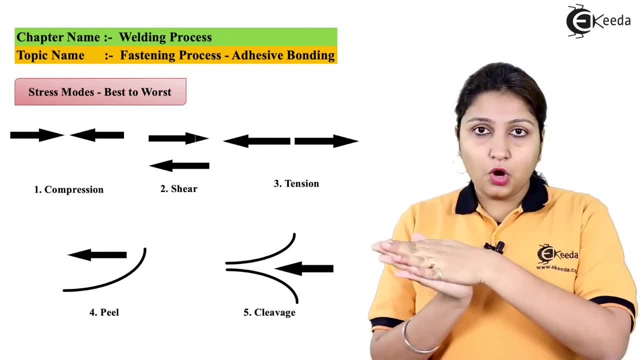 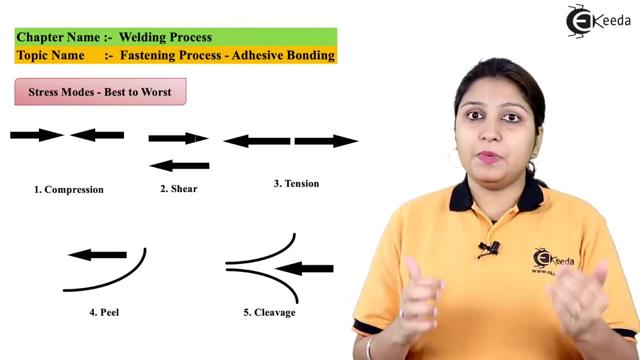 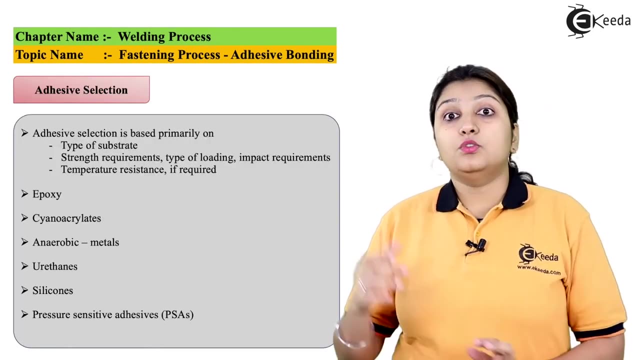 peeling. your object can be peeled, like if it is joined. you can peel and remove it, and the last part is cleavage. if your object is like this, the material can be pushed from between and it can be removed easily. so these are some kind of stresses which fall on your adhesive bonding. so these are